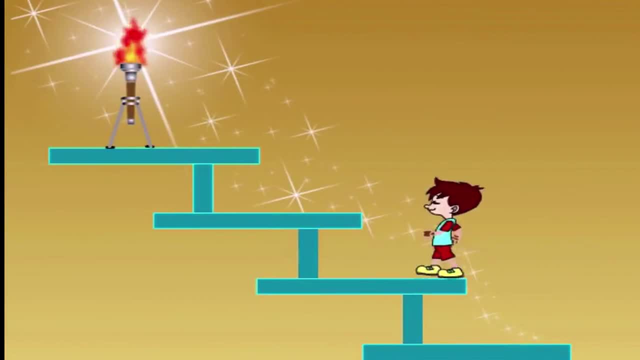 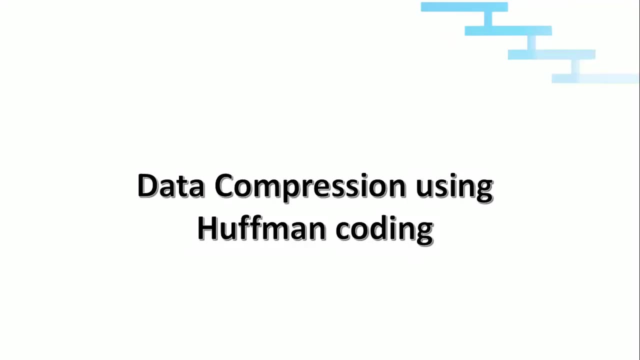 Hi guys, today we are going to see data compression using Uffman coding algorithm. The Uffman coding algorithm was invented by David Uffman in 1952.. The Uffman is particular type of optimal prefix code that is commonly used for lossless data compression. 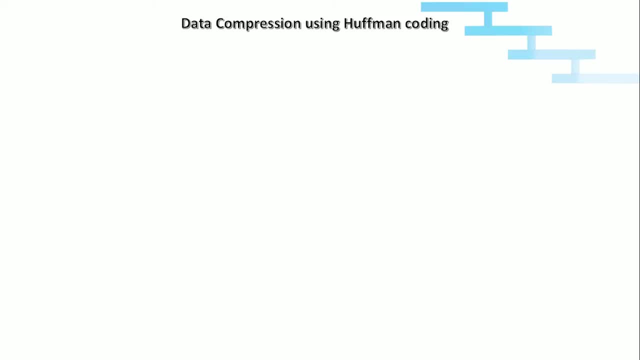 The thumb rule for the Uffman coding algorithm is: lesser the frequency, the greater the number of bits to represent the character. greater the frequency, lesser the number of bits to represent the character. We will see how this rule gets implemented in the Uffman coding algorithm. 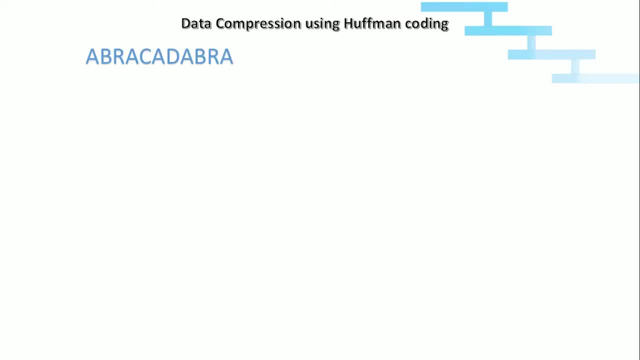 In this example we are going to compress the word abracadabra. The word abracadabra has 11 characters. if it takes 8 bits to denote each character, it will be taking 88 bits to encode abracadabra. Now we will compress this abracadabra using Uffman coding and we will see how much bits we can able. 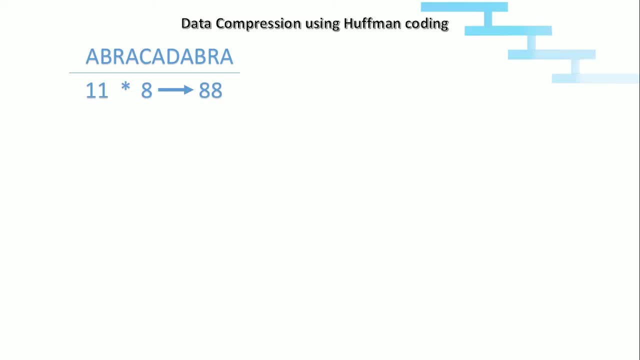 to reduce. First we need to count the frequency of each character in the given word. So we will take this word, abracadabra, and then, first, we will calculate the frequency of each character: a1, b, 1 r, 1 a, which is already 1, so it is 1 plus 1. c, 1 a, which is already 2. we include plus 1. 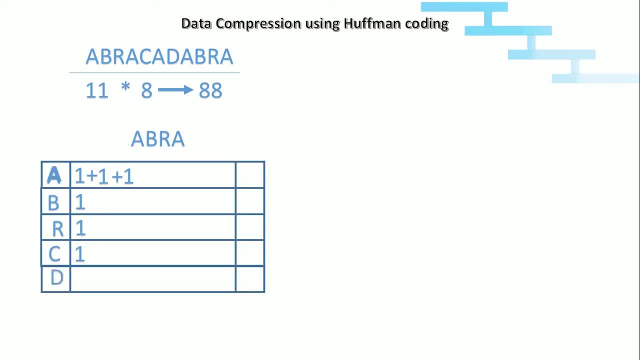 so 1 plus 1 plus 1. d, 1 and a, which is already 3, now we include plus 1. b, which is already 1, now include 1, so it will be 1 plus 1, now r, which is already 1, we will take 1 plus 1.. 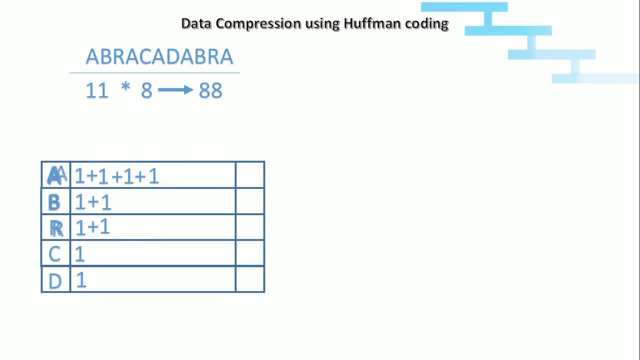 Now a, which is already four, we will take plus one, which will be five. Now we will get the total number of each character, which will be a5, b2, r2, c1 and d1.. We will count this 5 plus 2 plus 2 plus 1 plus 1, which will be 11.. 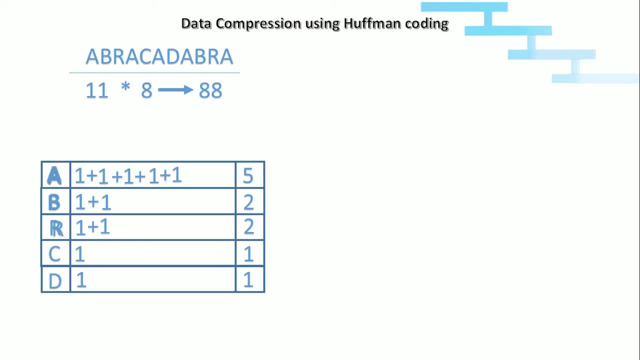 So we counted correctly. Now let's see how to compress data using Uffman coding. first rule is two characters, which has a lowest frequency. in our case, we have C with frequency 1 and the D with frequency 1, so we will take C and D, so we will. 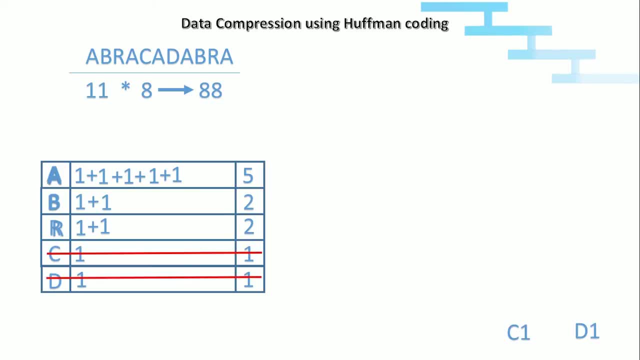 strike it off because we are taking it out now. we will create a relief root node with C 1 and D 1. the value of the root node is sum of the frequency of both nodes, that is, the sum of the frequency of C 1 and D 1, which will be 2. 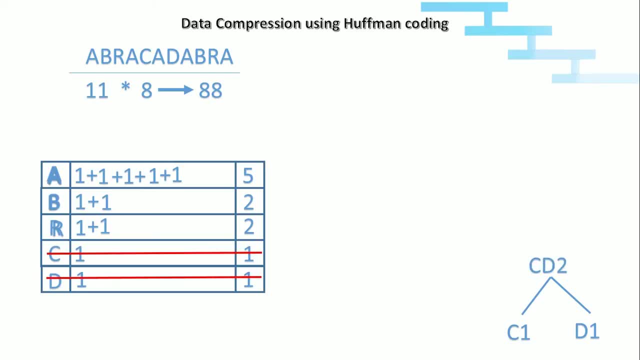 now we will check for the next lesser frequent character, which is R 2, and we will take the next lesser frequenter character, which is B. now we will form a root node. its value will be the sum of this B and R frequency, which will be 2. 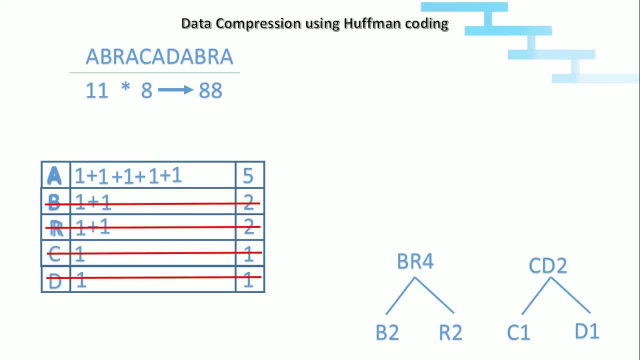 plus 2, which will be 4, and we will take the next lesser frequenter character. the next lower frequency is 5, so by comparing this, 4 can be joined with 2, because 4 and R are same, so they are the same. 5 are big when compared to 4 and 2, so we will merge 4 and 2, which will be 6, because b and r. 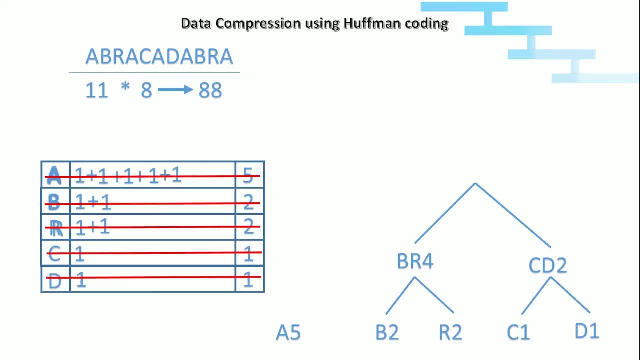 has a frequency 4, c and d has the frequency 2. so when combining all this, we will get the frequency 6.. now we will combine a's frequency and b or c, d, which frequency is 6. we will combine both this, the total frequency is 11.. always, the root node should match the number of characters in the word. 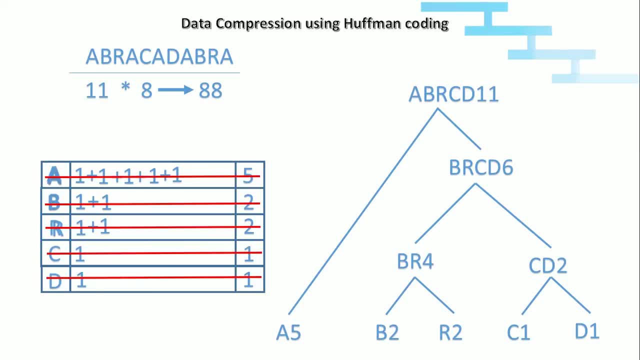 so our case, the root node value is 11, which is exactly matching with the number of characters, 11.. after that, we need to mention 0 to the left hand side and 1 to the right hand side, that is, 0 to the left hand side of the tree and 1 to the right hand side of the tree. we need to point all. 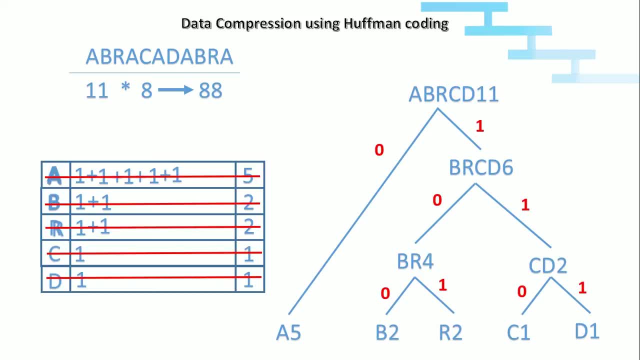 the edges like this, that is, that is, left branches in g and right branch is 1.. now we have computed the tree, now we need to find code for each and every character. for a it is 0 because it has only zero here, and for b it is 100 and for r it is 101. 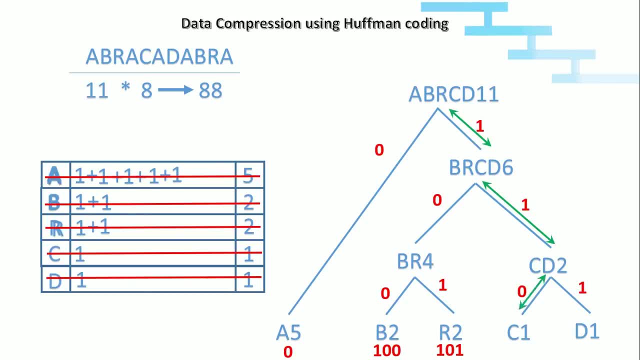 and for c it is 110 1 1 0 and for d it is 1 1 1. as we said earlier, the thumb rule: the higher the frequency, the lesser the number of bits to represent the character, in this case a, which is higher frequency it takes. 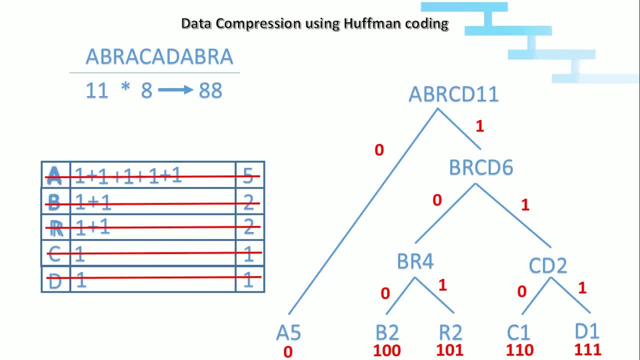 only one bit to represent d and all other characters, which has comparatively lesser frequency. it takes longer bits to represent. now we will compress the abracadabra with the code which we have found. so we wrote abracadabra. now replace all the a with 0. next we will take b. 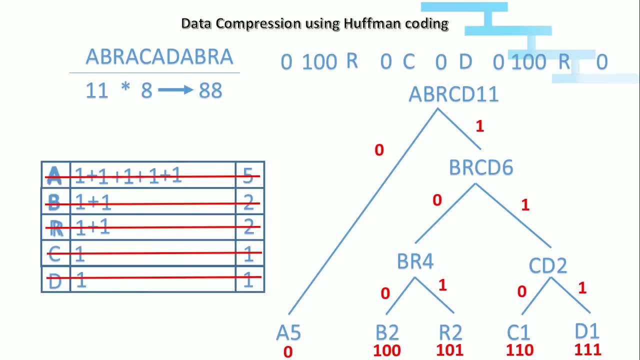 now replace all the b with 1 0 0. then replace all the r with 1 0 1. next replace all the c with 1 1 0. next replace d with 1 1 1. this is the compressed code which represents abracadabra now. 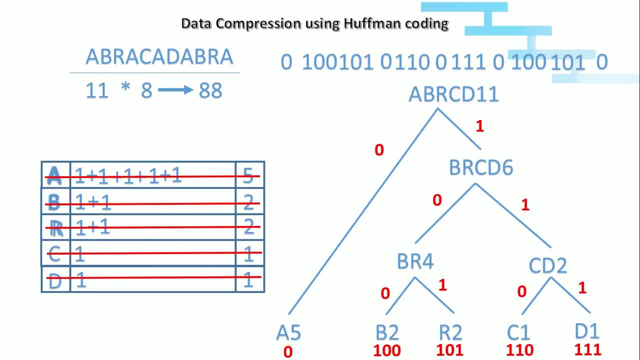 we will count the number of bits in the compressed code, which will be 23. so we found that if we compress with the regular methodology, it takes 8 bits to denote each and every character, which will be 88 bits by half one coding we have computed that it takes only 23 bits to denote. 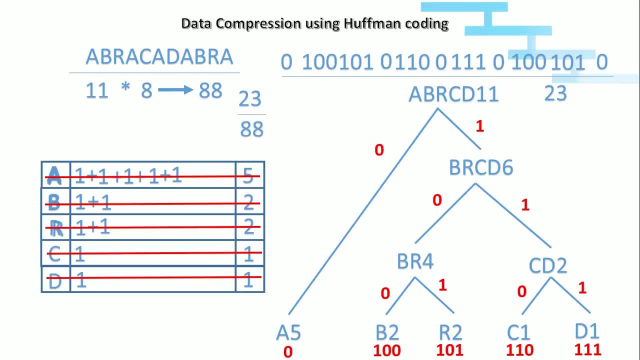 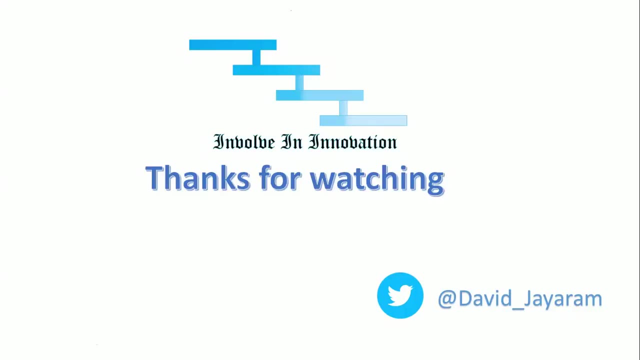 bits, so 23 divided by 88, which will be 26 percentage. we have reduced the code. now the compression percentage is 26 percentage, so by this way we can able to compress using halfman coding algorithm. thanks for watching this video. for more technical videos, please subscribe this channel.